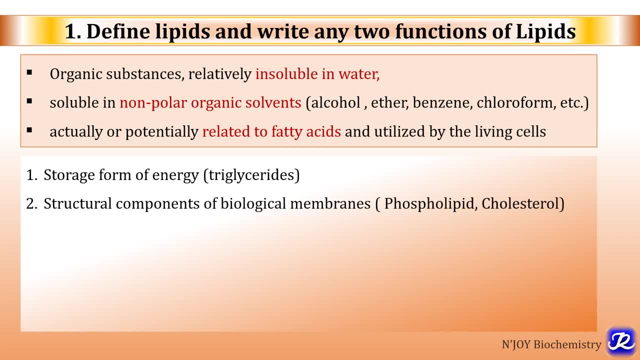 They are the structural components of biological membrane. So in the biological membrane it is made up of phospholipid bilayer and it also has cholesterol. It is a metabolic regulator, because the steroid hormones are derived from cholesterol, Likewise the prostaglandins, leukotrienes. they are also derived from arachidonic acid. 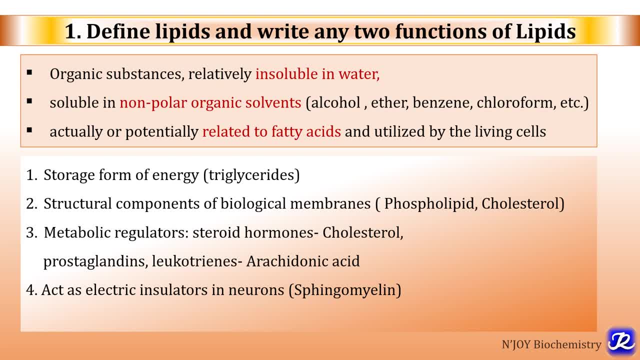 Then the lipids. they act as electric insulator in neurons- For example, sphingomyelin is electrical insulator- And lipids also protect internal organs due to the pads of fat, And they are also important for absorption of various fat soluble vitamins like A, D, E, K. 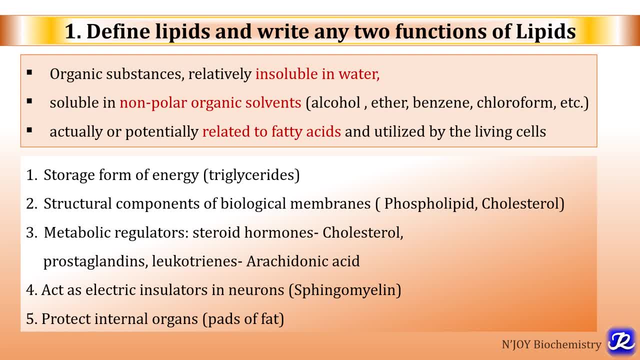 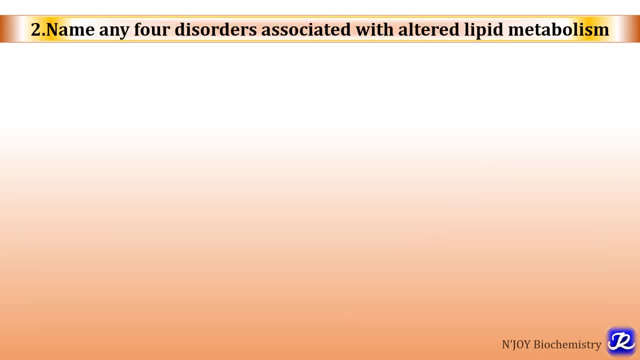 So there are various functions. out of those functions you can write any two functions of lipids. Second question is: name any four disorders associated with altered lipid metabolism. The answer is: obesity, atherosclerosis, diabetes mellitus, Fatty liver, familial hyperlipoproteinemia. 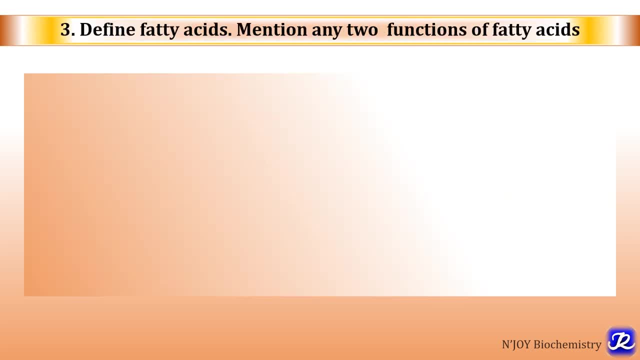 Question 3 is: define fatty acids. Mention any two functions of fatty acids. The definition is: fatty acids are long hydrocarbon side chain with carboxyl group at one end and methyl group at other end. So fatty acids are the carboxylic acid with hydrocarbon side chain. 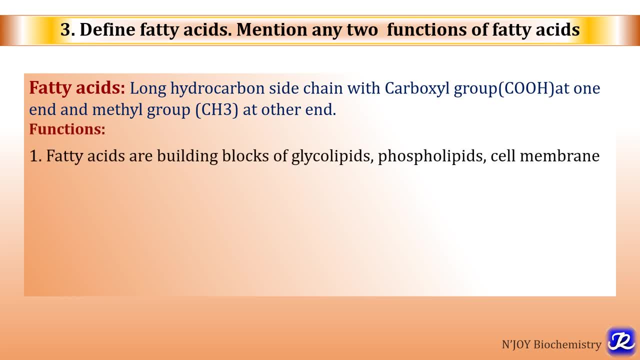 The functions of fatty acids are: they are the building blocks of glycogen, Glycolipids, which contains lipid plus carbohydrates, phospholipids and cell membrane. Second function is fatty acid, for example, arachidonic acid. It is a precursor of eicosanoids, and the examples of eicosanoids are prostaglandins, lipoxins, leukotrienes. 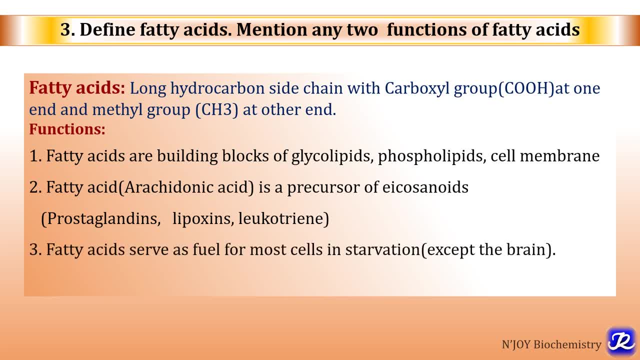 This is the second function. Third function is fatty acids serve as fuel for most of the cells in starvation, except the brain, Because fatty acid cannot cross blood brain barrier. Fatty acids are stored in the form of TAG, that is, triglycerides in adipose tissue. 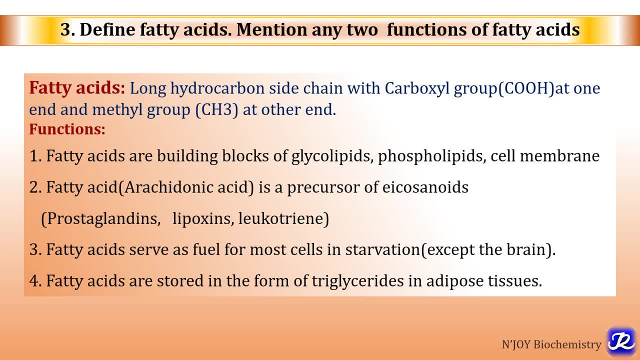 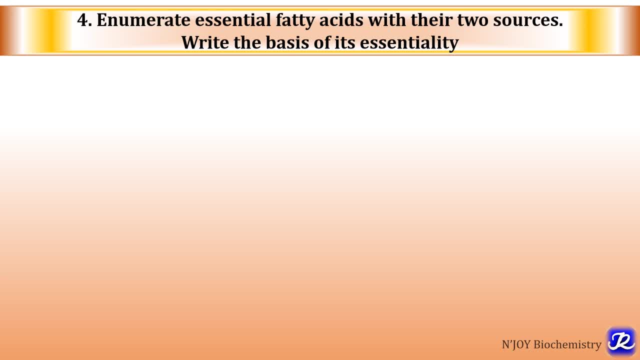 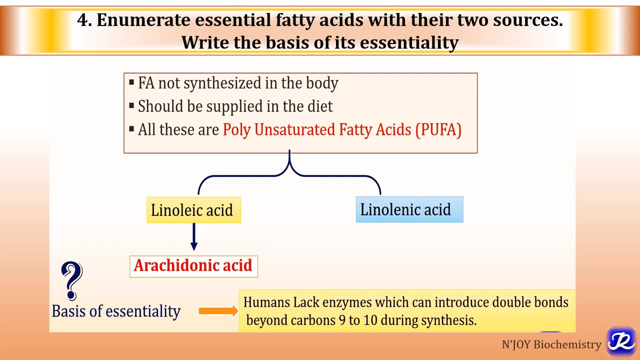 So these are the various functions out of which you have to write any two functions of fatty acids. Fourth question is: enumerate essential fatty acids with their two sources and write the basis of their essentiality. So the examples of essential fatty acids are linoleic acid and linoleic acid. 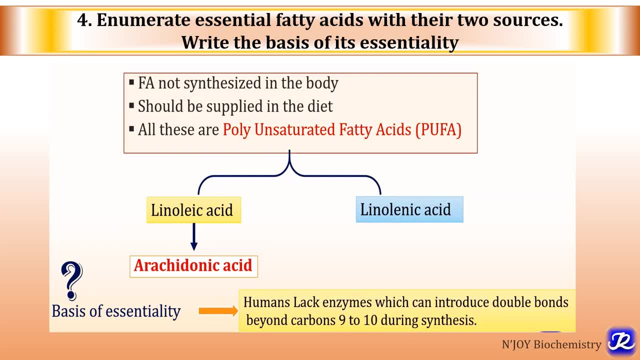 Arachidonic acid is derived from linoleic acid, So it is not considered as essential fatty acid. Essential fatty acid means the fatty acids which are not synthesized in the body and should be supplied in the diet, And all the essential fatty acids are polyunsaturated fatty acids which contain double bonds. 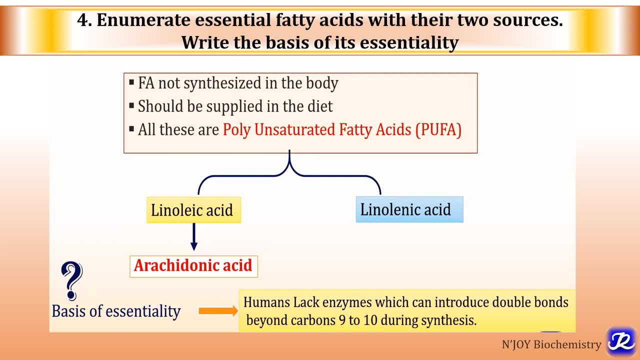 And what is the basis of their essentiality? Humans lack enzymes which can introduce double bonds beyond carbon 9 to 10 during their synthesis, And both these linoleic and linoleic- they have double bond beyond carbon 9.. So that's why they are essential. they cannot be synthesized in the body. 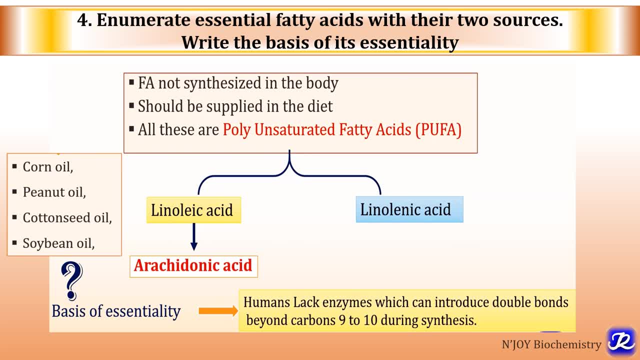 And the sources of linoleic is corn oil, peanut oil, cottonseed oil, soya bean oil, And linoleic sources are walnut oil, flaxseed oil, canola oil, fish liver. So these are the various sources. 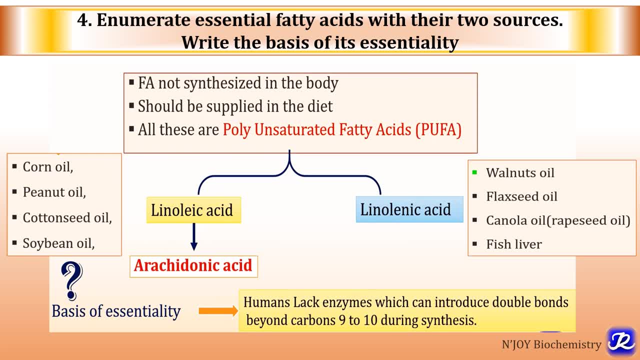 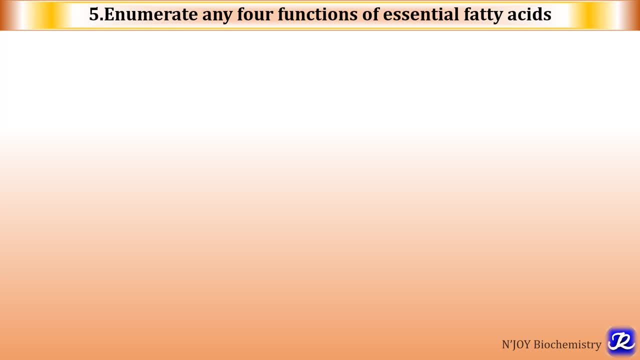 So you can write any two of the sources and the essential fatty acids. its basis of essentiality should be mentioned. Fifth question: enumerate any four functions Of essential fatty acids. So first is, as arachidonic acid is derived from linoleic acid, which is the essential fatty acid, 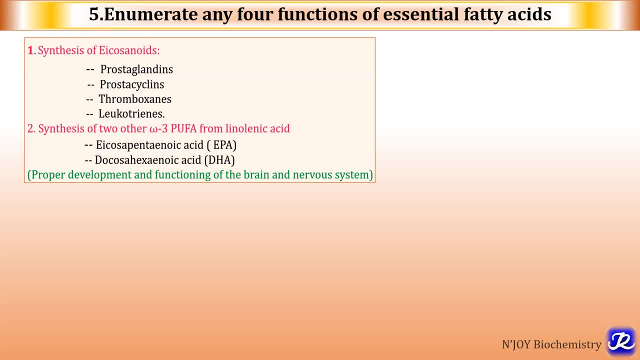 And that arachidonic acid is involved in the synthesis of eicosanoids like prostaglandins, prostacyclines, thromboxane and leukotrienes. So this is the first function: Synthesis of two other omega 3 PUFA from linoleic acid. 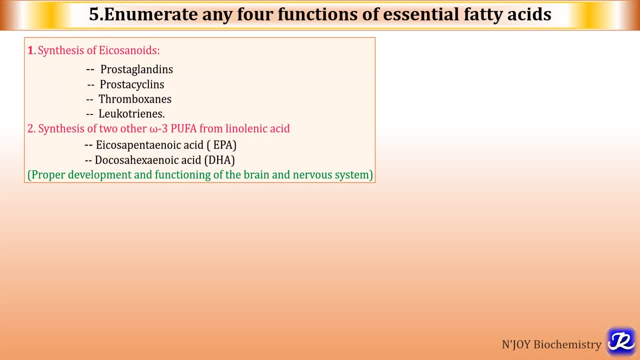 So from the linoleic acid, the eicosapentaenoic acid and docosahexoanoic acid, which is required for the progesterone, Proper development and functioning of brain and nervous system, is synthesized, And that's why this is the second function of essential fatty acid. 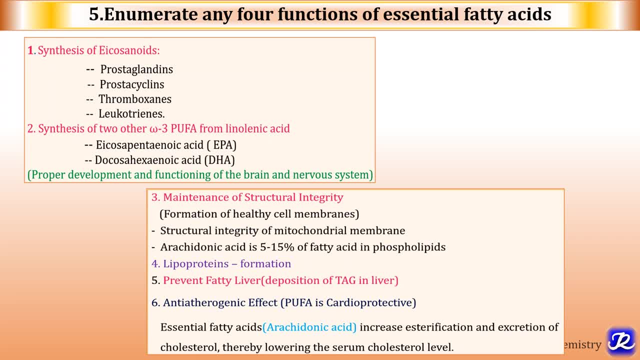 Now these essential fatty acids. they are required for maintenance of structural integrity, formation of healthy cell membrane and also the mitochondrial membrane. Because the arachidonic acid, which is derived from linoleic acid, it is 5 to 15% of fatty acid in phospholipid. 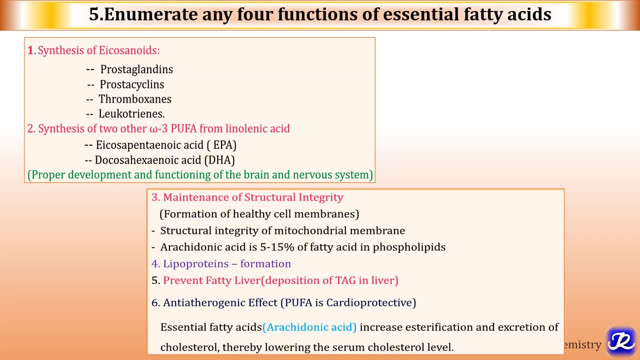 And they are also involved in the lipoprotein, Because lipoprotein has single phospholipid layer and phospholipid they have arachidonic acid. Then fifth function is the essential fatty acid. they prevent fatty liver, They have anti-athrogenic effect and that's why it is called PUFA is cardioprotective. 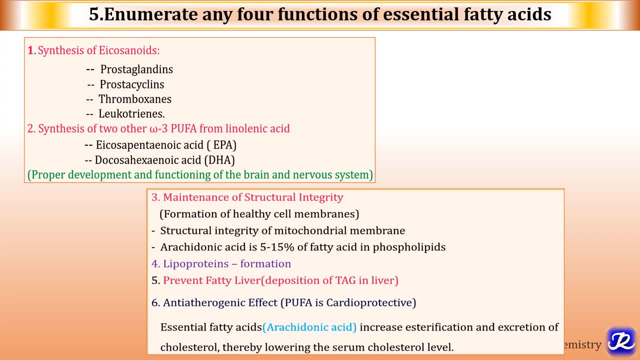 Now this PUFA here is arachidonic acid. Because this essential fatty acid, arachidonic acid, it increase esterification and excretion of cholesterol And thus it lowers the serum cholesterol And it is involved in reverse cholesterol transport. So these are the various functions of essential fatty acid, out of which you can write any four functions. 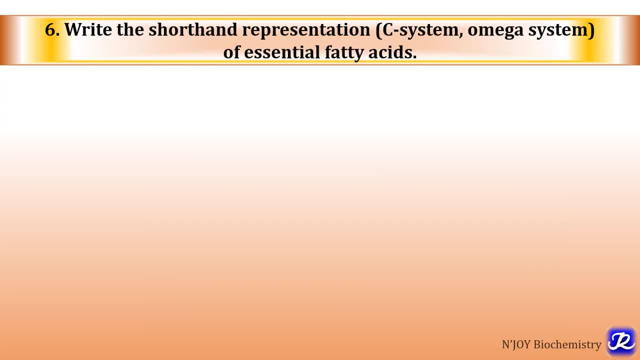 Sixth question is write the shorthand representation that is in the C system and omega system of essential fatty acid. So linoleic acid is the essential fatty acid. In the C system it is written as C18 2 because there are two double bond delta 9, 12.. 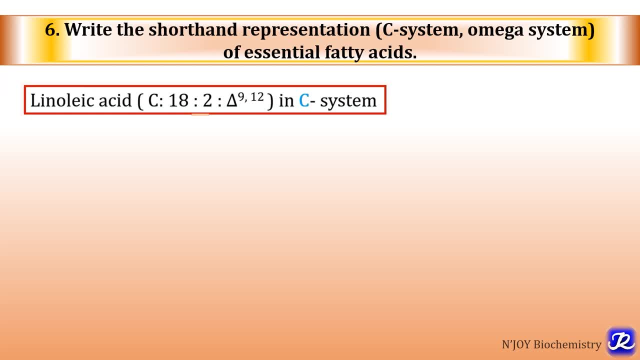 So first double bond Is between carbon atom 9 and 10 and second double bond is between carbon atom 12 and 13.. So in the C system it is written like this: In the omega system, linoleic acid is written like C18, because 18 carbons are there. 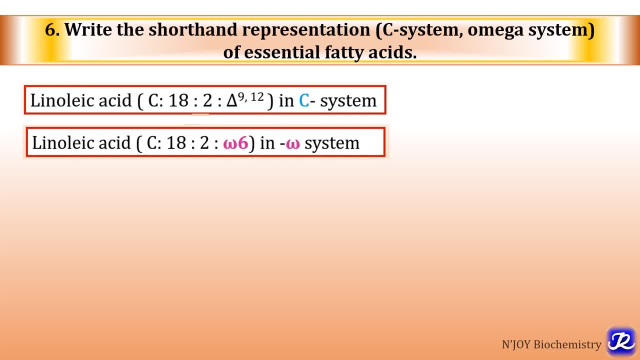 2 because two double bonds and omega 6 because the first double bond is between omega 6 and 7 carbon Linolenic acid. it also has 18 carbon. but there are three double bonds. First double bond is between 9- 10.. 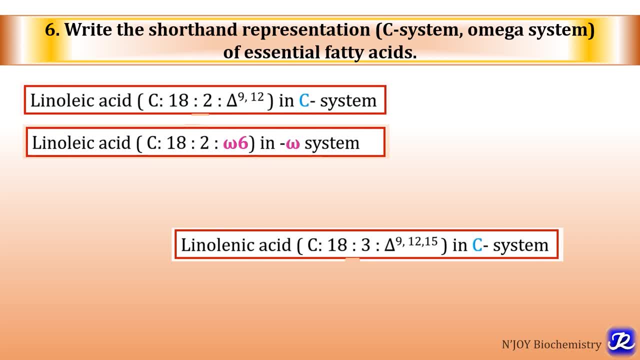 Second double bond is between 9- 10.. Third double bond is between 12- 13 carbon and third, between 15 and 16 carbon. So that's why it is written as C18, 3 delta, 9, 12 and 15 in the C system. 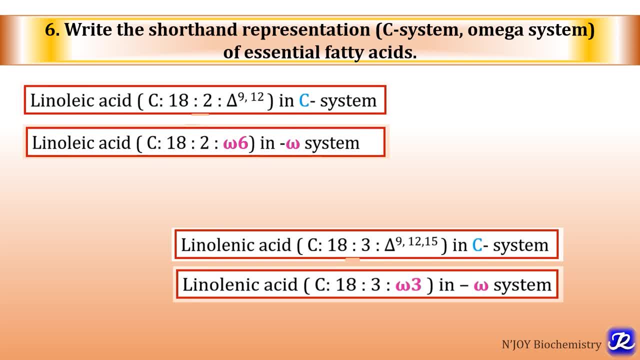 While in the omega system C18 3, because three double bond, but first double bond is between omega carbon 3 and 4.. That's why it is C18 3, omega 3.. So this is how the essential fatty acids, like linoleic acid and linoleic acid, they are represented. 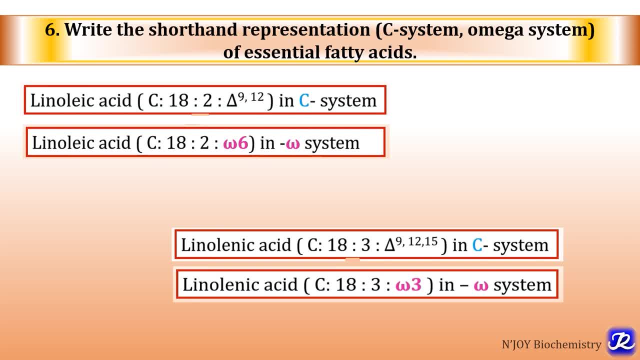 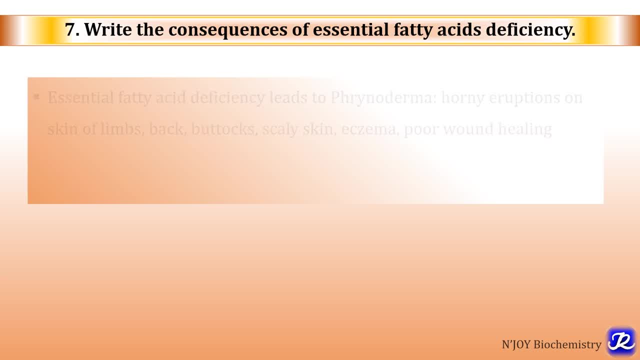 In both C system and omega system. Seventh question is: write the consequences of essential fatty acid deficiency. So if there is essential fatty acid deficiency it leads to the condition called as phrenoderma, or toad skin. There is horny eruptions on skin of limbs, back, buttocks. 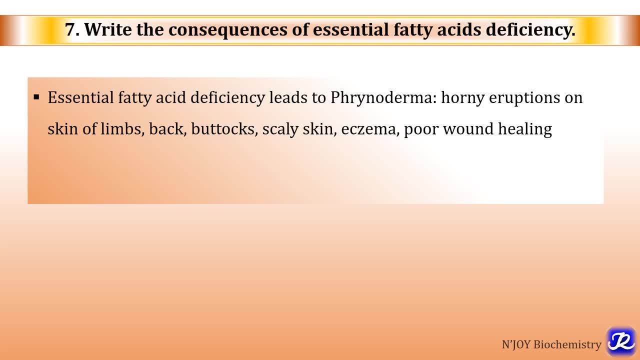 There is scaly skin, eczema, and it is also characterized by poor wound healing. Now the essential fatty acid deficiency can also lead to The lipid transport and also the fatty liver. it decreases the efficiency of biological oxidation, because essential fatty acids are required for the structural integrity of mitochondrial membrane. 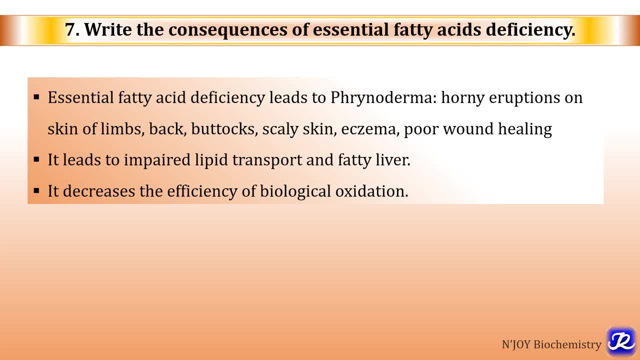 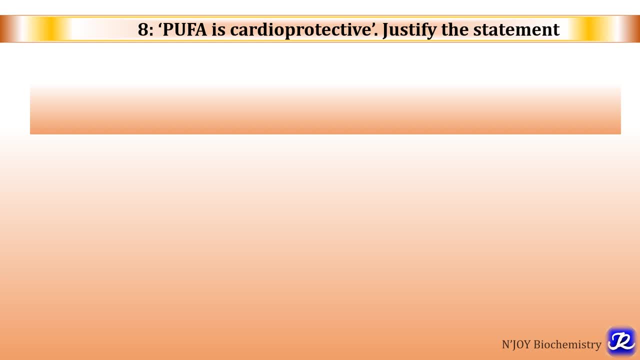 So these are the various consequences of essential fatty acid deficiency. Eighth question is: PUFA is cardioprotective. justify the statement here. PUFA means arachidonic acid, that is, polyunsaturated fatty acid. Arachidonic acid is the constituent of phospholipids. 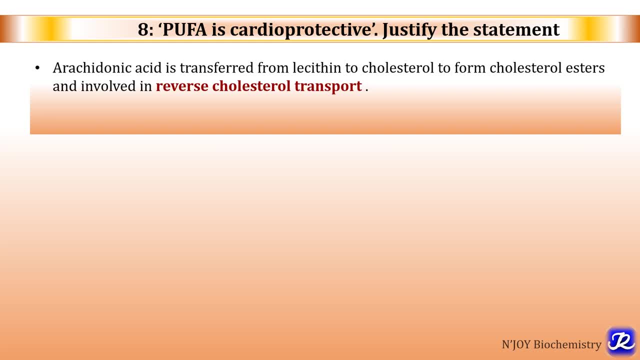 That is phosphatidylcholine, which is also called as lecithin. There is transfer of this arachidonic acid from lecithin to the cholesterol and there is formation of cholesterol esters, And this is sterification process is very important in the reverse cholesterol transport. 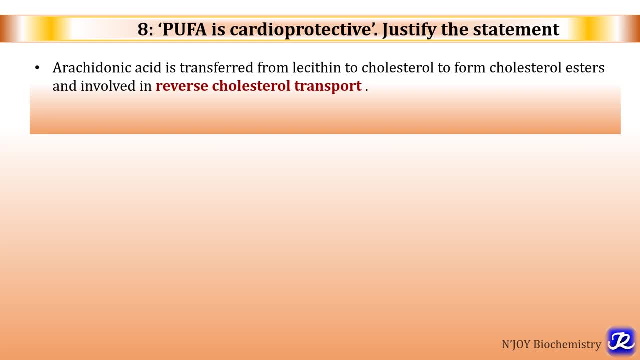 That is, transport of cholesterol from peripheral tissues to the liver and it is carried out by the lipoprotein HDL, that is, high density lipoprotein. So because of this is sterification, there is more Uptake of cholesterol from the peripheral tissues and then that cholesterol is delivered from the peripheral tissues to the liver for metabolism and thus it leads to decrease in the serum cholesterol level. and this is anti-arachidonic effect, where the arachidonic acid plays very important role, and that's why it is said that PUFA is cardioprotective. 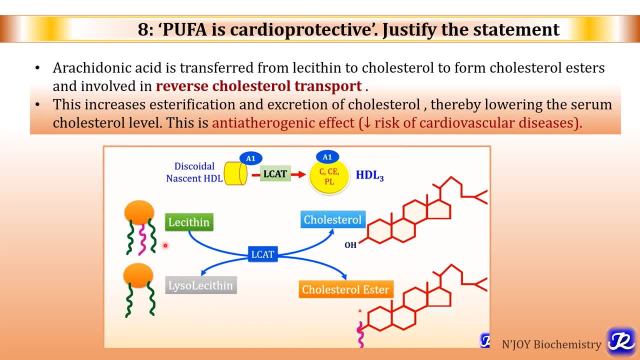 So the arachidonic acid. from lecithin. it goes to cholesterol to form cholesterol esters By the action of enzyme lecithin cholesterol acyl transferase and because of this is sterification. the discoidal nascent HDL becomes mature, spherical HDL3 and it plays important role in reverse cholesterol transport. and reverse cholesterol transport is very important because it has the anti-arachidonic effect, as HDL carries cholesterol from peripheral tissues to liver and that's why it is said that PUFA is cardioprotective. 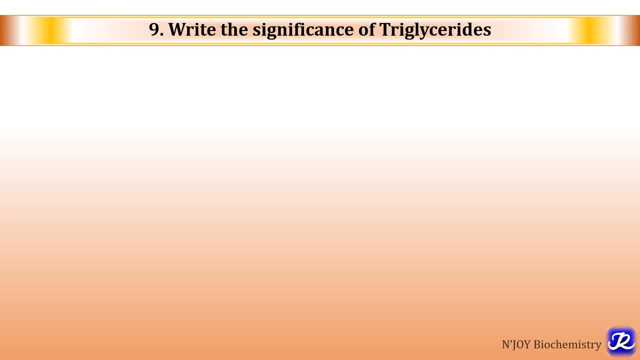 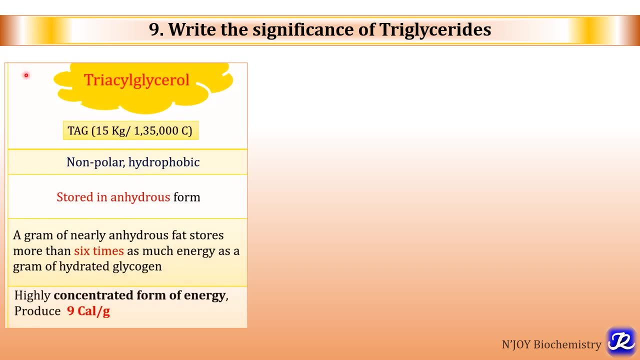 Ninth question is: write the significance of triglycerides. Triglycerides are the neutral fats and it is the simple lipid. It is the storage form of lipid and the fatty acids are stored in the form of triacylglycerol in adipose tissue. 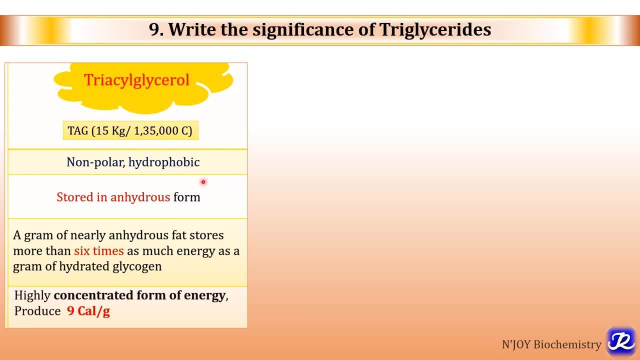 These are nonpolar, hydrophobic and they are stored in the anhydrous form, and it is the highly concentrated form of energy which produces 9 kilocalorie per gram, and a gram of nearly anhydrous fat stores More than 6 times as much energy as a gram of hydrated glycogen. 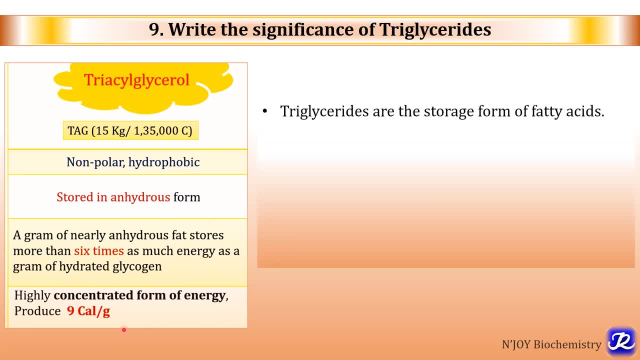 So triglyceride, it is the storage form of fatty acid. it is highly concentrated form of energy and in fasting and starvation triglycerides are broken down, that lipolysis, which is a lysis or breakdown of triglycerol into glycerol and fatty acid, and this process occurs under the influence of glucagon in fasting and starvation. 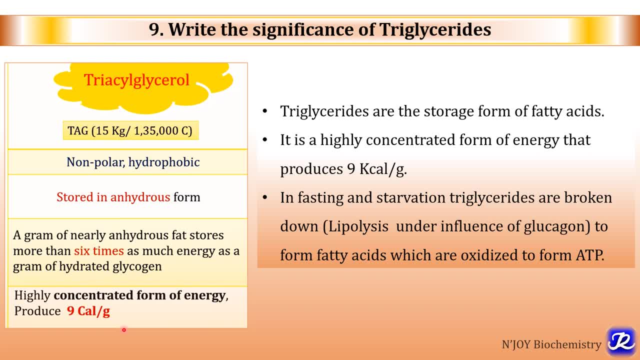 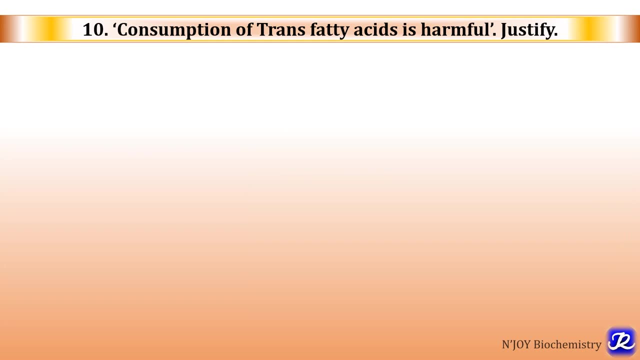 And the fatty acid which are produced By lipolysis. they undergo beta oxidation and to form ATP. So that's why the triglycerides are important. Question number 10 is: consumption of trans fatty acids is harmful. Justify Now, the trans fatty acids are unsaturated fatty acid in the trans isomeric form and these are produced by fermentation in human of dairy animals and also by catalytic hydrogenation of vegetable oil. 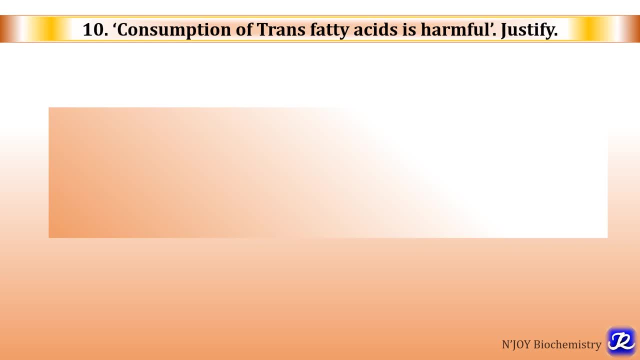 And various sources are dairy products, meat, fried food, cookies, etc. Now we will see why the consumption of trans fatty acid is harmful, Because they compete with essential fatty acid and causes essential fatty acid deficiency. They increase THG level, LDL level and thus leads to increased risk of cardiovascular diseases. 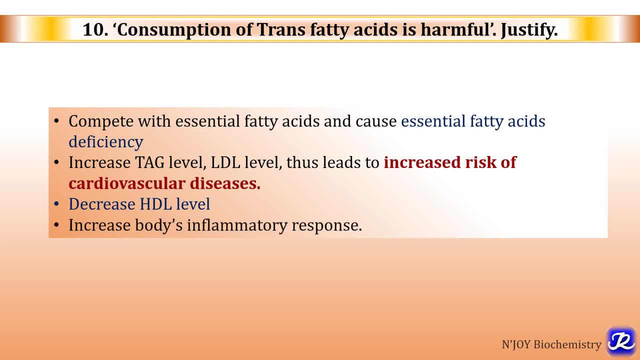 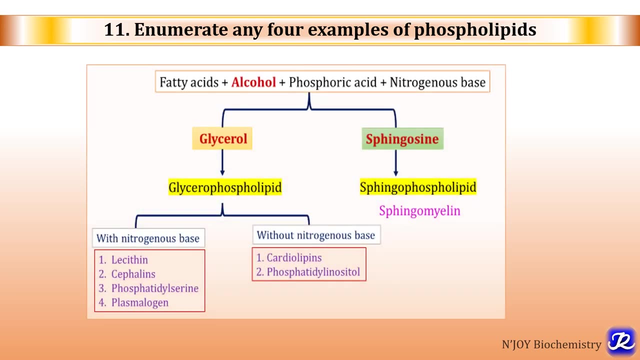 They decrease the HDL level and increase body's inflammatory response, And that's why it is said That consumption of trans fatty acid is harmful. Enumerate any four examples of phospholipids. Phospholipids are the compound lipids which are made up of fatty acid plus alcohol, plus phosphoric acid, plus nitrogenous base. 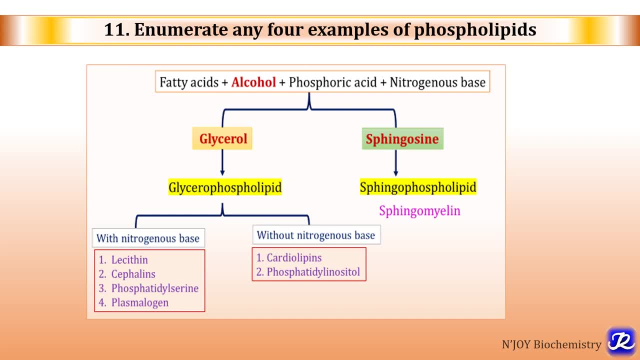 Now, depending upon the alcohol present in the phospholipid, they are again classified as a glycerophospholipid. if glycerol is the alcohol and sphingophospholipid is, sphingosine is the alcohol in phospholipid. 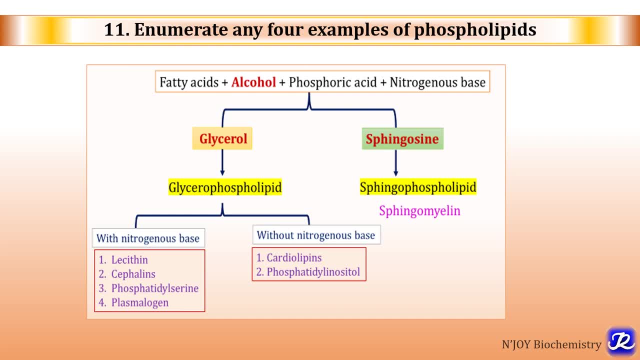 Now glycerophospholipid with nitrogen. Nitrogenous base are lecithin, cephalin, phosphatidylserine, plasmalogen and glycerophospholipid without nitrogenous base are cardiolipins, phosphatidyl, inositol and sphingomyelin is sphingophospholipid. 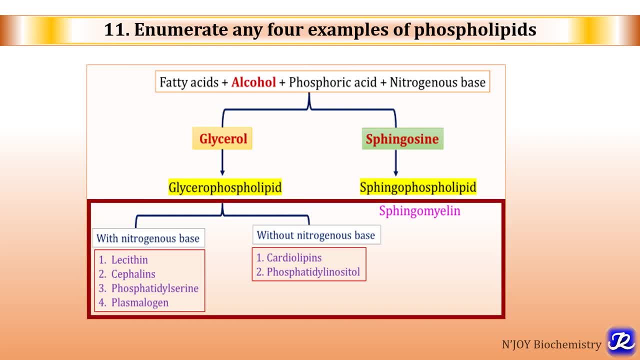 So the question is: enumerate any four examples of phospholipids. So you can just enumerate the examples like lecithin, cephalin, phosphatidylserine, plasmalogen, cardiolipin, phosphatidyl inositol and sphingomyelin. 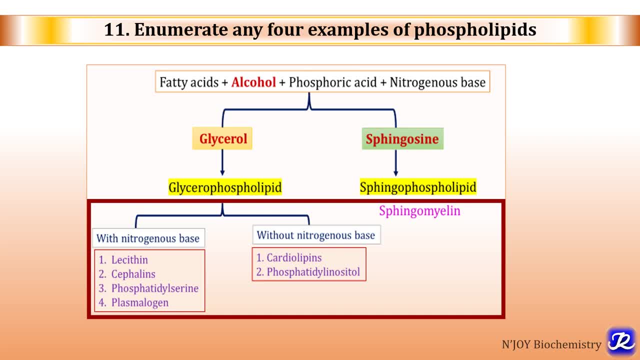 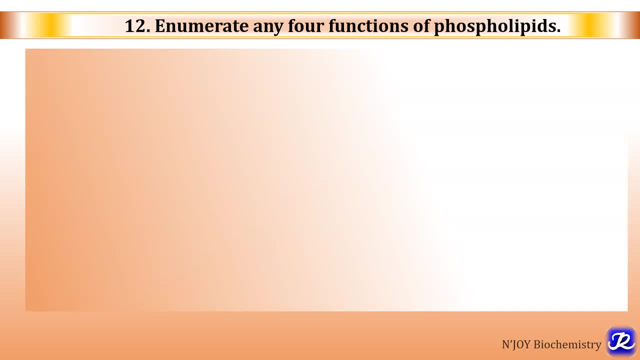 So out of this you can Enumerate any four examples. Enumerate any four functions of phospholipids. Phospholipids play very important functions. They are the major lipid constituent of cellular membrane, because cellular membrane is made up of phospholipid bilayer. 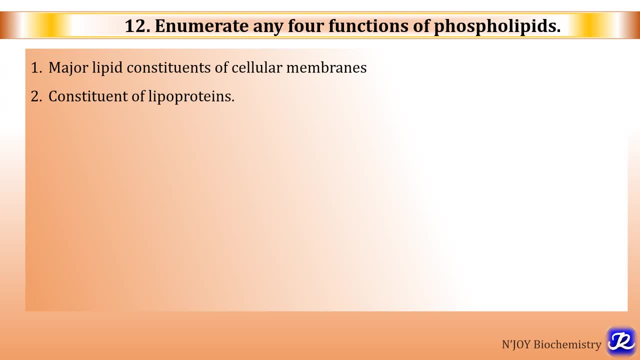 Constituent of lipoprotein. lipoprotein membrane is a single layer made up of phospholipid and cholesterol Lecithin, which is also called as phosphatidylcholine. It represents a storage form of lipotrophic factors like choline and methyl group. 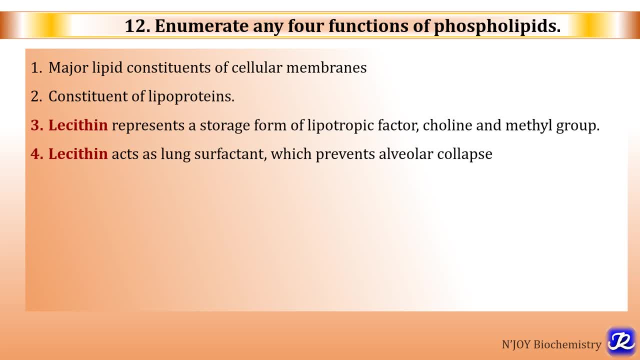 Lecithin also acts as lung surfactant, which prevents alveolar collapse. Dipometyl lecithin Thromboplastin, which is also called as a coagulation factor 3.. It is composed of mainly important phospholipid, that is, cephalin. 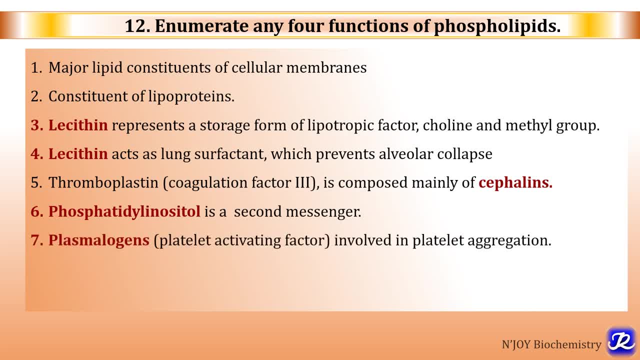 Phosphatidyl inositol is a second messenger, Plasmalogen, which is also called as platelet activator. Plasmalogen is 엑 soundedist Breadlet factor. It is involved in platelet aggregation. Sphingomyelin act as electrical insulator around. 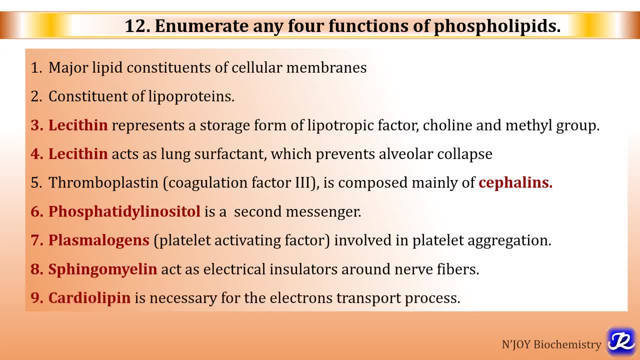 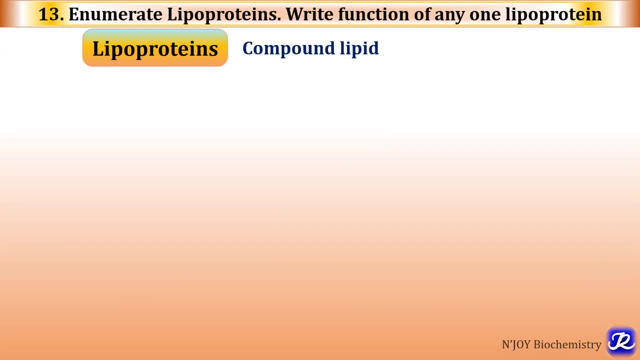 the nerve fibers. Cardiolipin is necessary for electron transport process, So there are many functions of phospholipid Here. you have to write any four functions and this topic is very important for SAQ also. Next question is: enumerate lipoproteins and write. 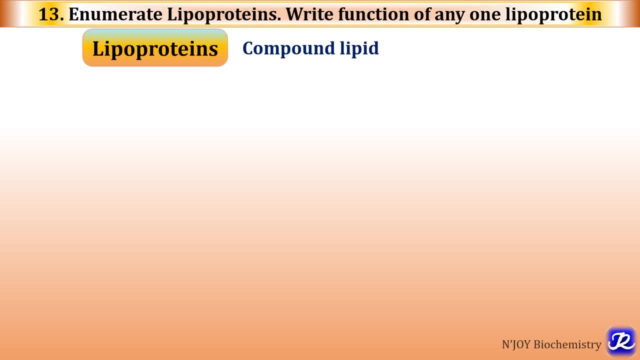 function of any one lipoprotein. Lipoproteins are the compound lipids, So the lipoproteins are chylomicrons, very low density lipoprotein, low density lipoprotein, intermediate density lipoprotein and high density lipoprotein. So here you have to enumerate the lipoproteins. 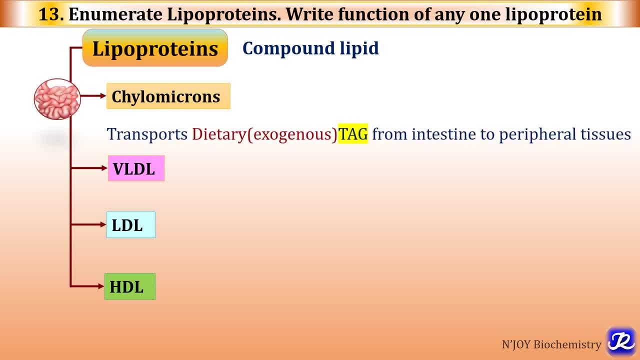 Now the chylomicrons. What is the function of chylomicron? Chylomicron is synthesized in the intestine and it transports dietary or exogenous triglyceride from the intestine to the liver. So this is the function of the lipoprotein. So here you have to enumerate. 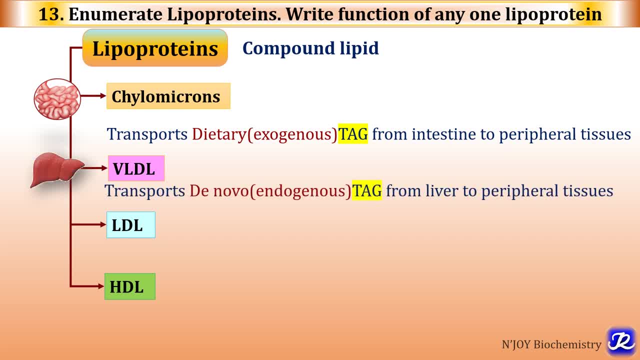 to peripheral tissue. This is the function of chylomicron VLDL. it is synthesized in the liver and it is involved in the DNO, or endogenous triglyceride transport from the liver to peripheral tissue. So this is the function of VLDL, that is, it carries triglyceride from liver to 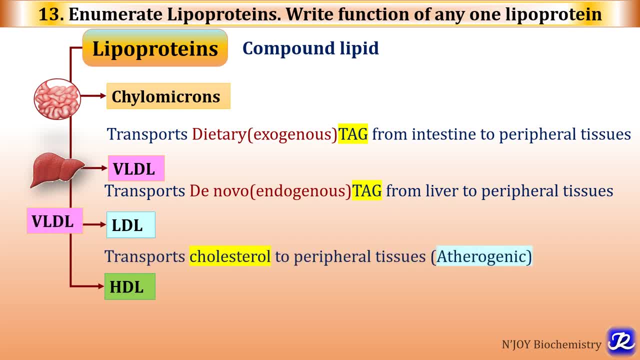 peripheral tissue. Now, what is the function of LDL? LDL is derived from VLDL in the circulation and it transports cholesterol to the peripheral tissue and that's why it is called as atherogenic and HDL. it is synthesized from intestine and liver and it transports cholesterol from peripheral 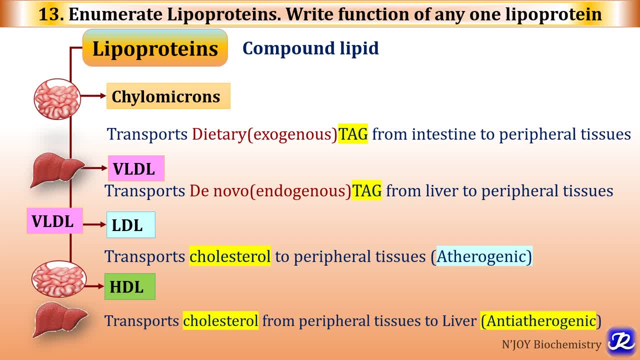 tissues to liver. that is reverse cholesterol transport and that's why HDL is called as anti-atherogenic. So here you have to enumerate the names of lipoproteins and you can write any function of any one lipoprotein. the function you can write the function of chylomicron. 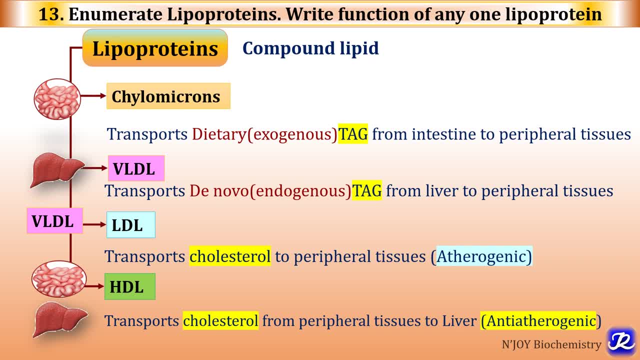 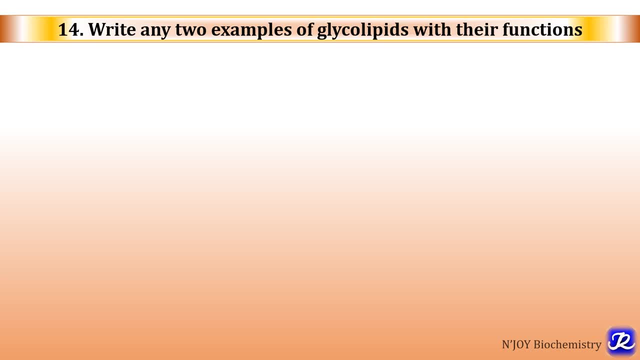 VLDL, LDL or HDL? 14th question is: write any two examples of glycolipids with their functions. Glycolipids are also compound lipids. The examples are cerebroside, sulfatides, globosides and. 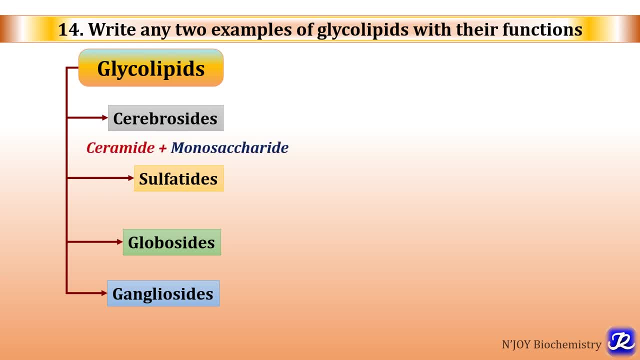 gangliosides. Cerebrosides are made up of ceramide plus monosaccharide, and the galactocerebroside is present in the nerve tissue membrane. Glucocerebroside is present in non-neural tissues. 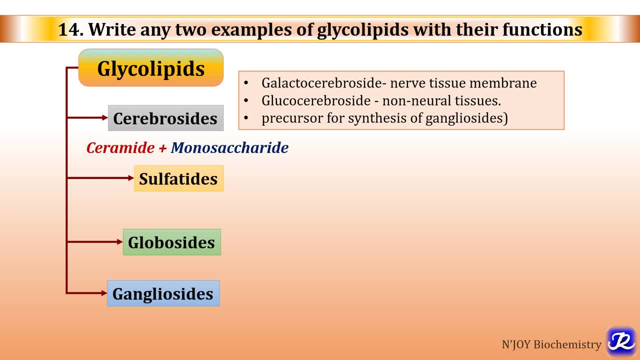 and they are also involved in the synthesis of glycol. So this is the function of glycol. This is of gangliosides, more complex glycolipids and sulfatides. contains ceramide plus monosaccharide plus sulfur and sulfogalactoceramide. it is found in the myelin Globosides made up of ceramide plus. 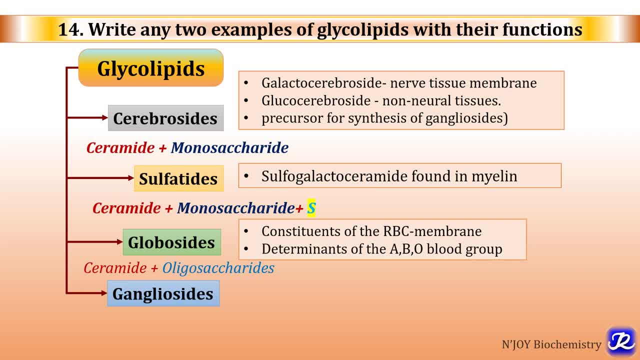 oligosaccharides, and they are the constituent of RBC membrane and determinants of ABO blood group Gangliosides. they are made up of ceramide plus oligosaccharides plus nana, that is N-acetyl acid. So these are the various examples of glycol lipids Here. you need not to write composition, you have. 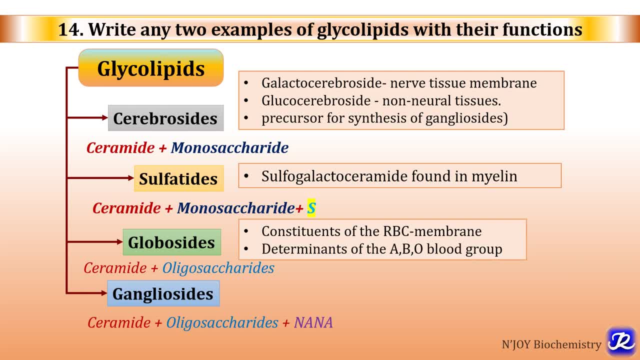 to write any two examples, like cerebrosides, sulfatides, and you can write their function. For example, galactocerebroside- it is involved in the formation of nerve tissue membrane, and glucocerebroside, present in the non-neural tissues, and sulfogalactoside ceramide, found in the myelin.